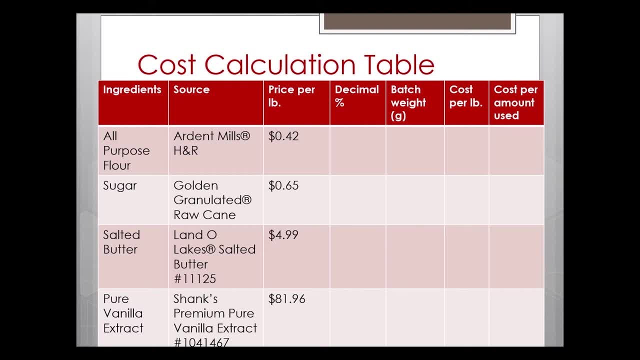 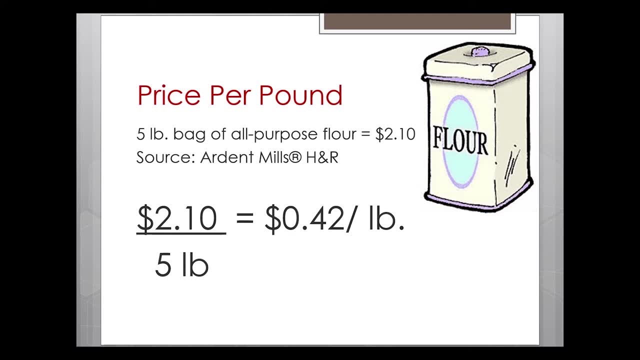 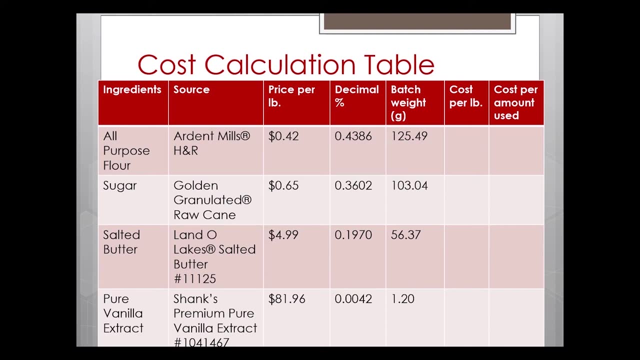 This is obtained from your supplier or from the store prices that you have been using. If the bag of flour is sold in five pound bags, divide the price of that ingredient by five to obtain the price per pound. Next, the weight percentage of the recipe and the batch weight are added into the table. 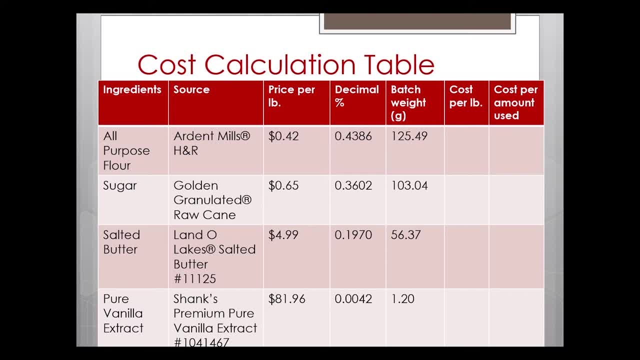 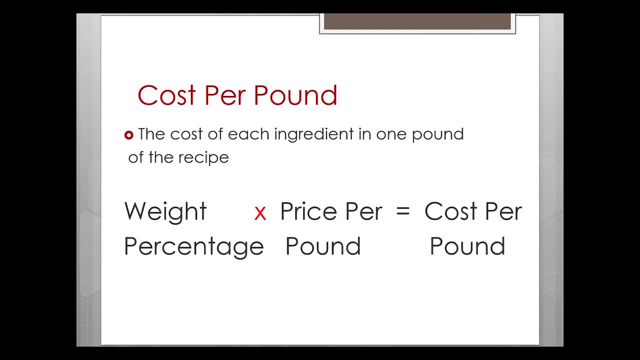 The batch weight is the amount of ingredient being used in the particular batch being made. The weight percentages should have been calculated prior to the formation of the cost calculation table. Then the cost per pound value must be calculated. Cost per pound is the cost of the particular ingredient in one pound of the full recipe batch. 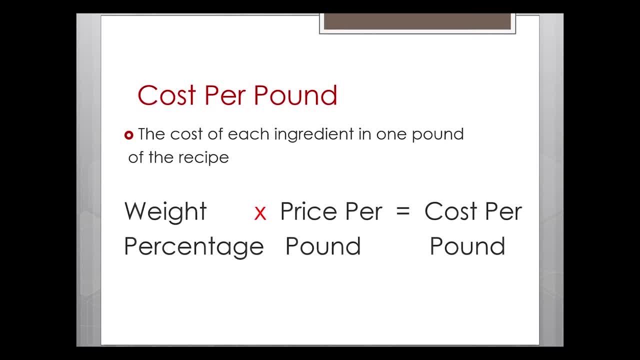 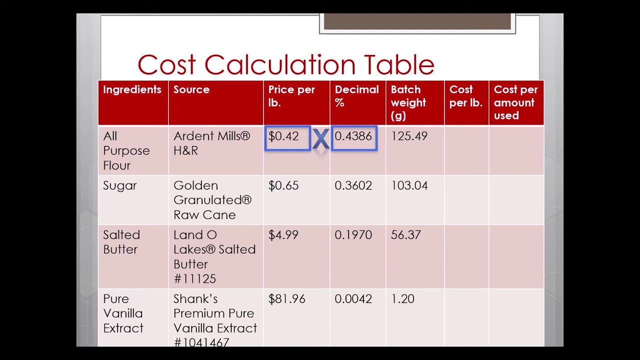 This value is calculated by multiplying the ingredient price per pound by the formula weight percentage. This value is then divided by 100.. In this example, 42 cents, which is the price per pound of flour, is multiplied by the weight percentage, which is 43.86%. 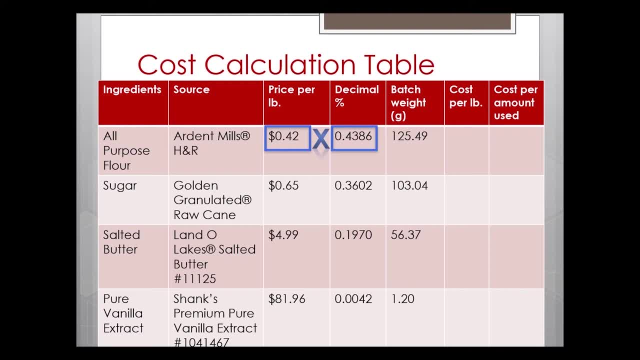 The product is then divided by 100, making the cost per pound recipe 18 cents. These steps were repeated for each ingredient. The final column in our cost calculation table is the cost per amount used. This column depends on the batch weight for each ingredient. 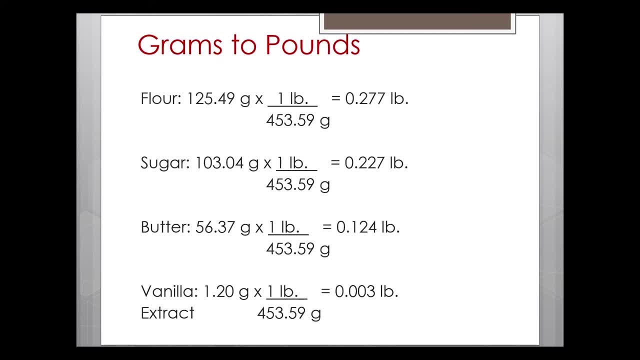 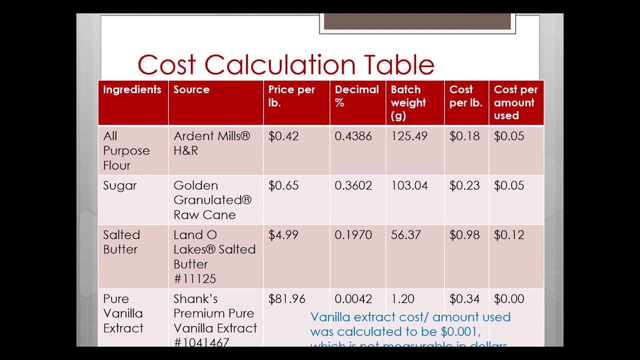 The batch weight should be converted to pounds through the simple unit conversion techniques shown here. The batch weight value in pounds is then multiplied by the cost per pound. Notice how vanilla extract seems to cost 0 dollars and 0 cents. This is due to the very small batch size. 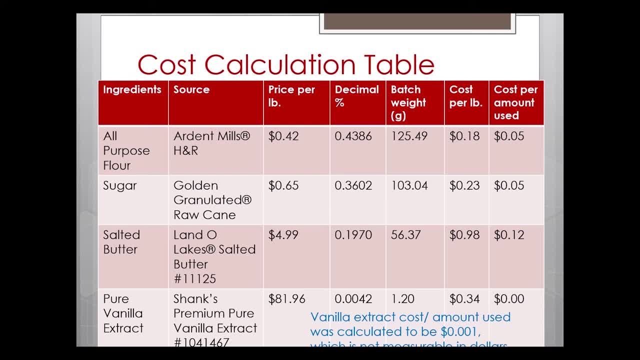 When this recipe is scaled up, the cost per amount used will increase as well. The final step to completing the cost calculation is to take the sum or the total of the cost per amount used. The total cost for the particular batch size shown in this example. 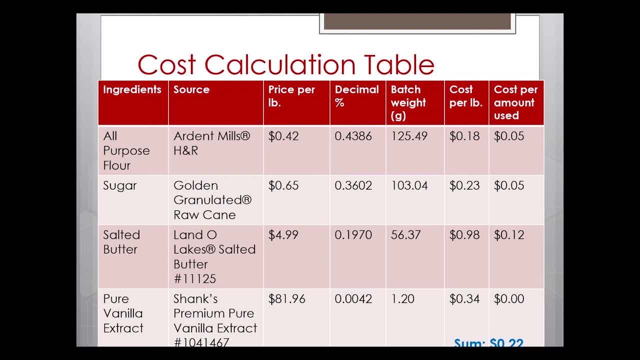 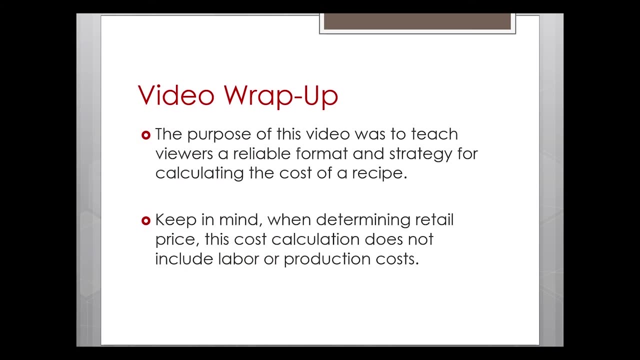 was 22 cents. The total cost per pound is also a helpful value to be aware of. After adding the values together, the cost per pound of this recipe is 1 dollar and 73 cents. In today's video, we learned a reliable table format for calculating the cost of a recipe. 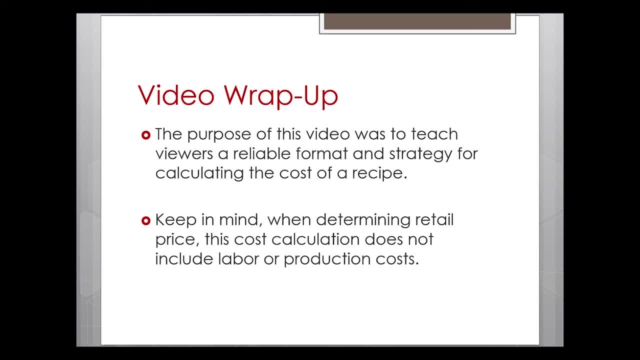 The purpose of this video was to highlight the factors that determine ingredient cost When determining retail price for your product. be mindful that this calculation is based strictly on the ingredients and does not include the labor facility or distribution costs of your product. Thank you for joining us today and good luck with your ingredient cost calculations. 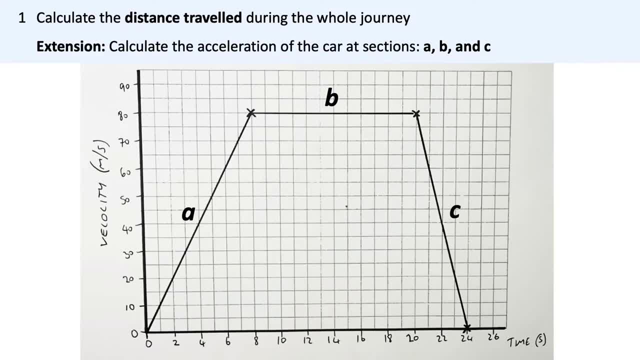 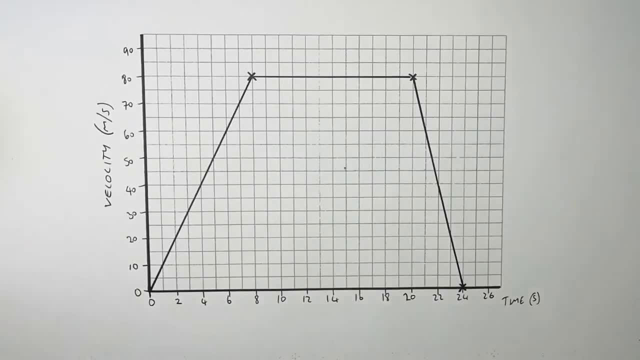 This is the problem. you will learn how to solve. Press pause to attempt it. The method and the answer will follow. So to calculate the distance a car has travelled using a velocity time graph, you must calculate the area underneath the lines, underneath the 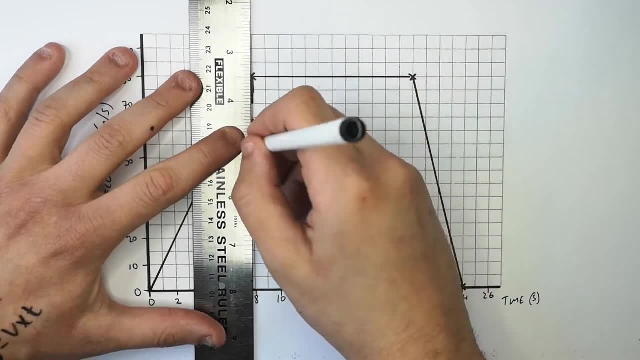 graph. So you must first identify where you can separate the graph into triangles, rectangles or squares. And that's what I've done here. I've split my graph into two triangles and one rectangle, So to calculate the distance the car travelled while the car was accelerating. 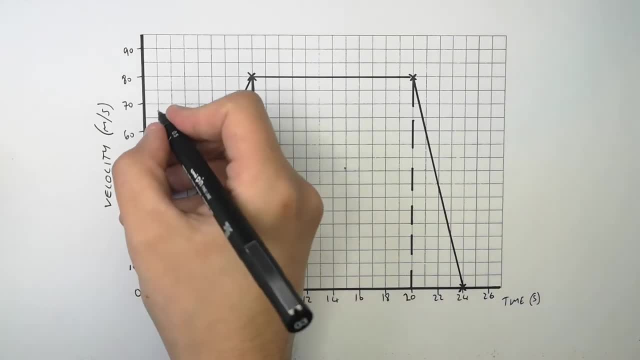 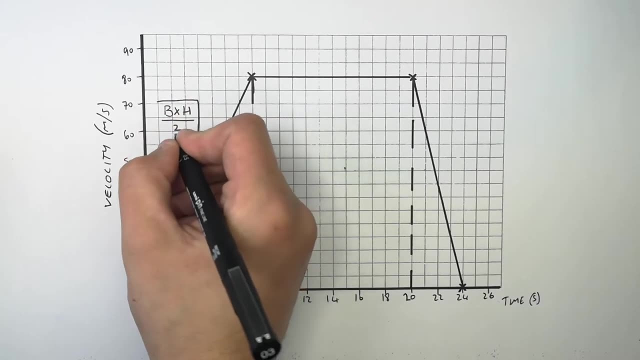 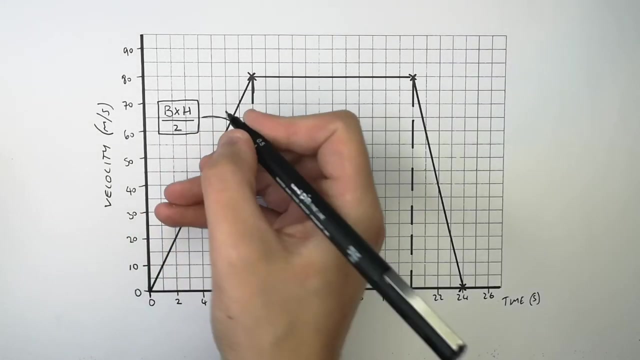 you must calculate the area of the triangle. And to calculate the area of a triangle you use the equation base times height divided by 2. That will give you the area in this triangle. So to calculate the area we must first identify the base and the height of the triangle. And to 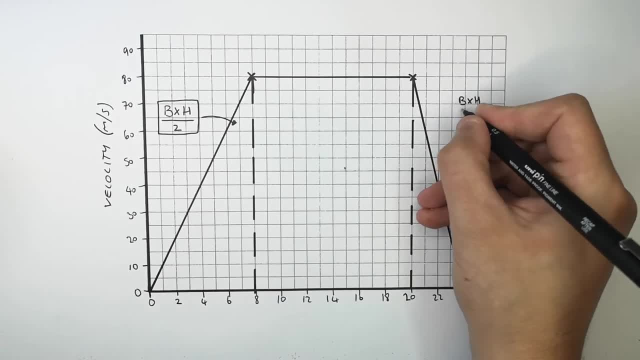 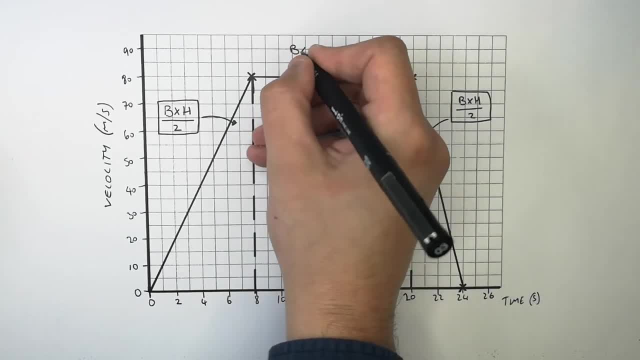 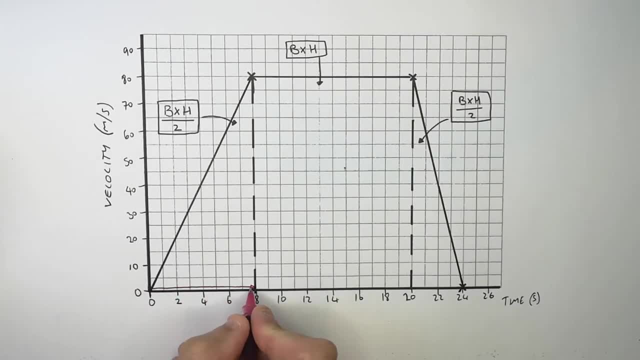 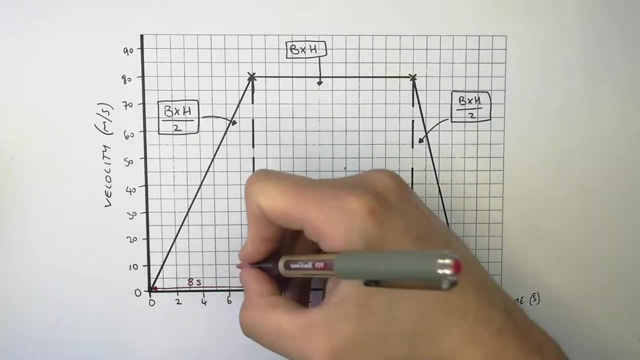 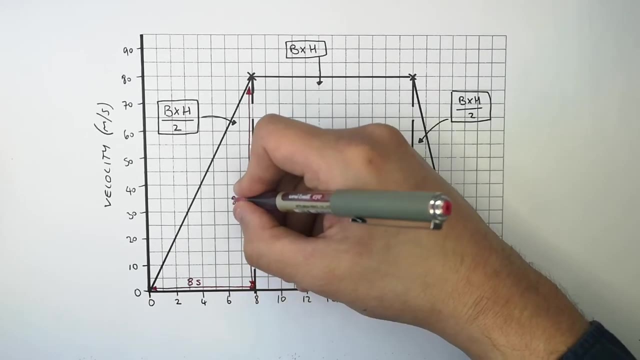 equation: base times height divided by 2, so you must identify the base. This is going to be 8 seconds, so b equals 8.. Then to work out the height of the triangle, that's going to be the velocity change, so that is going to be 80 meters. 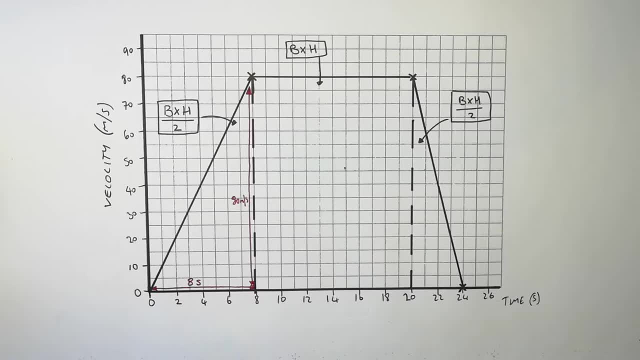 per second. So now you've got the base and the height. you simply do base of 8 times height of 80 and consider the triangle, divide it by 2 and that will give you a distance the car traveled of 320 meters. So the car travelled 320 meters in the